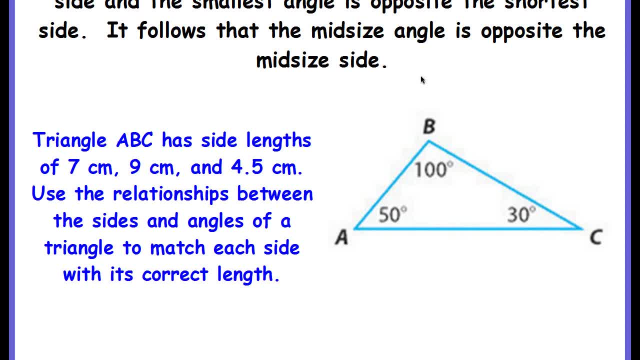 opposite the mid-sized side. Okay, so what it's saying is that the large angle is opposite the large side, or the longest side, The smallest angle is opposite this smallest side and the middle angle is opposite the middle size. Think of it as going to McDonald's and ordering an extra value meal You can get. 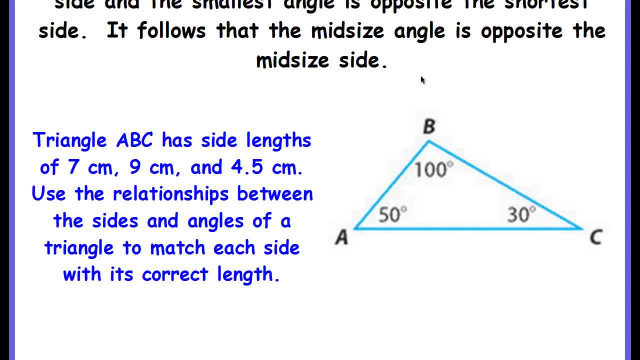 the small size where it comes with the small fries and the small drink. You can get the the middle size where it comes with a middle size and the smallest size. You can get the middle size where it comes with a medium french fry and a medium drink. or you can get the large size where you get 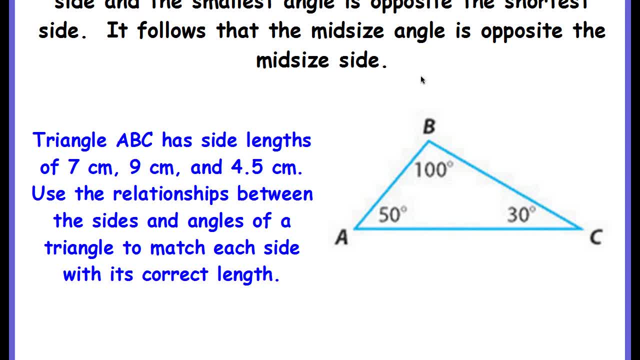 the large size, the large french fries and a large drink. Okay, so we have a triangle here and we're given three of its angles and it tells us that triangle ABC has side lengths of seven centimeters, nine centimeters and four and five tenths centimeters. We're going to use this relationship of small side. 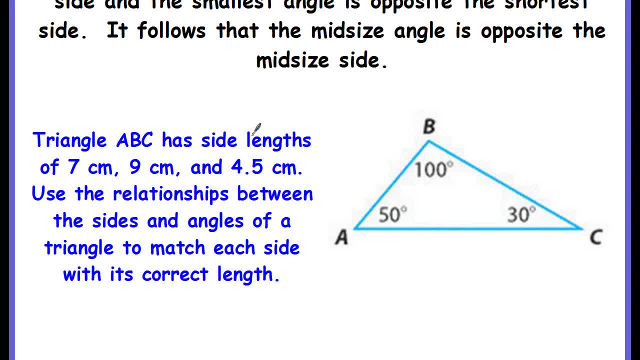 opposite small angle, etc. to match the side. each side with its correct length. Alright, so let's take a look. First of all, let's start. I always like to start with a large. You don't have to start with a large, but I'm going to start with. 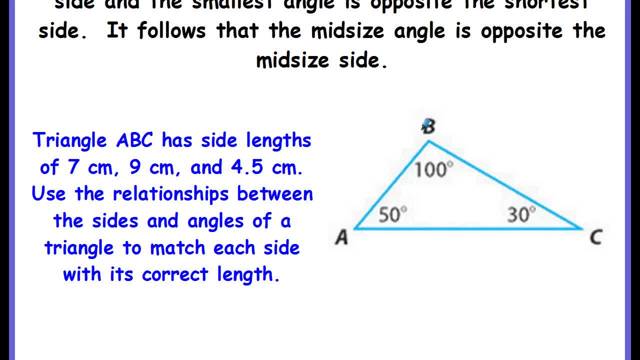 a large and the largest angle is going to be angle B at a hundred degrees. Now I need to know the side that is opposite this angle. This one's pretty easy to tell. Sometimes they're a little difficult to tell, So general rule is: 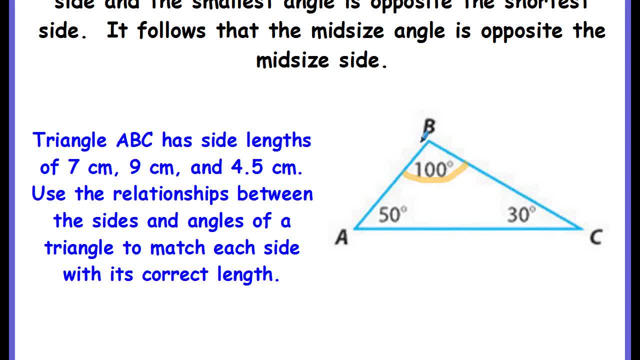 that it's the side that does not touch the angle. So here's my angle right here And if you look this, side AB and side BC, they both touch angle B, but angle AC does not. So this is the side that is opposite angle B, and since angle B is, 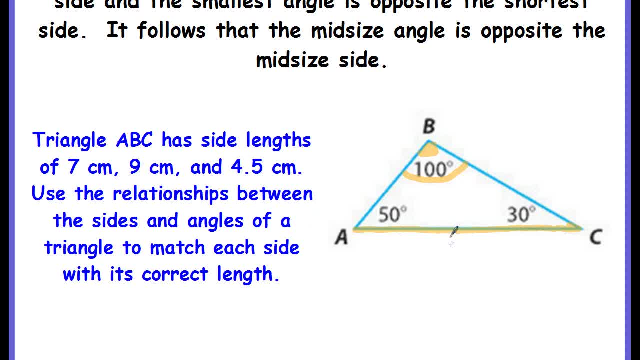 the largest angle. we want the largest side length to go here, and the largest side is nine centimeters, So this would be nine centimeters. Okay, let's go on to the next one. Let's go for the smallest. This 30 degrees is the smallest. 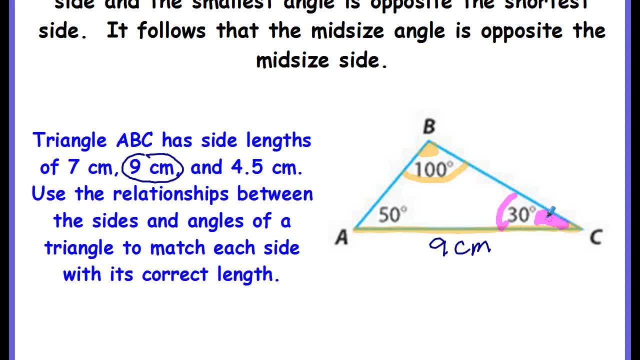 angle. so C is your smallest angle and we want the side that is opposite C. again. it's the side that does not touch C. AC touches C, BC touches C, but AB does not. So this is the side that is opposite angle C, and since angle C is the 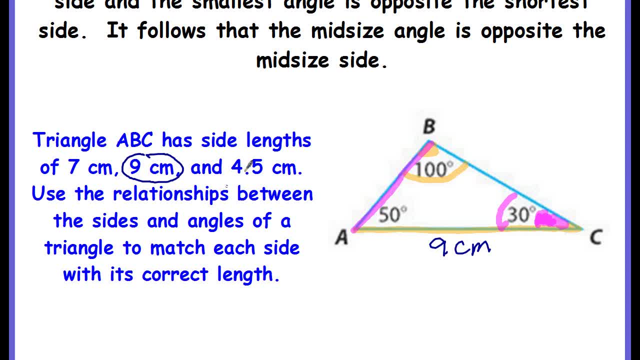 smallest angle. at 30 degrees, we want the smallest side or the shortest side, which is the 4.5 centimeters, And then it follows that the remaining ones are going to be the ones that are opposite. So we have angle A. this is the middle or the medium size angle and the only side that 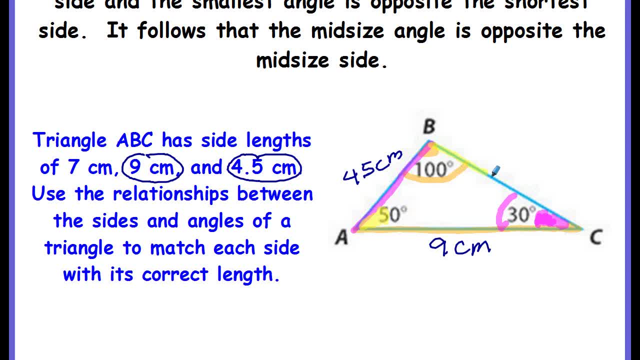 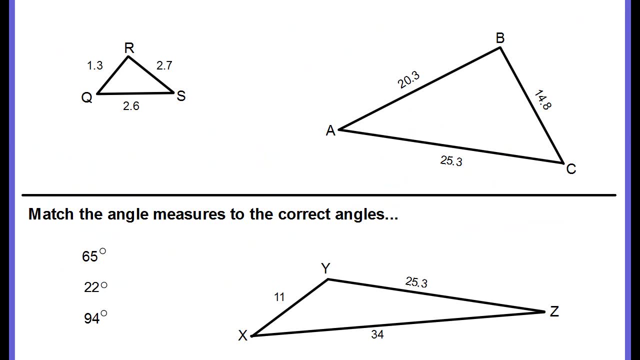 it doesn't touch or that doesn't touch. angle A is BC, So this is the opposite side, And we're going middle to middle, 7 centimeters, And that's all there is to it. So for each triangle, we're going to list the angles in order of smallest to greatest. 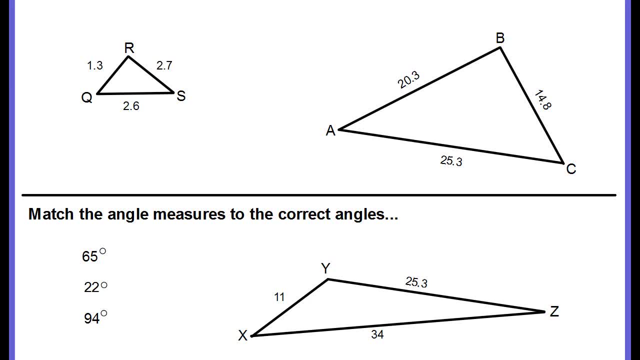 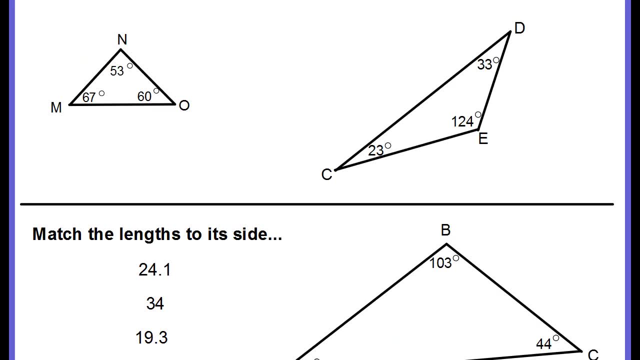 Okay. Okay, I think my pages got out of order, so hold on just a second. let me change them up for you. There we go. this is better. We're going to list the sides in order of longest to shortest And again we're given the degrees. 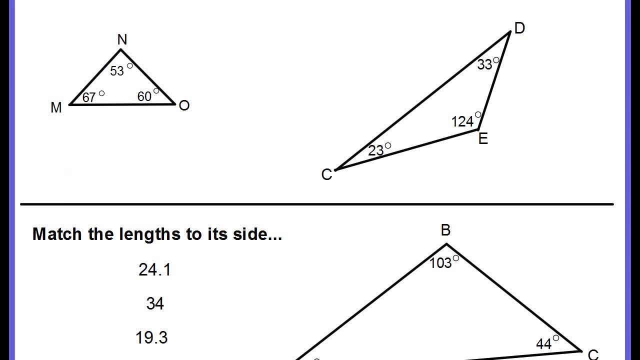 So let's start with the longest. longest goes with largest. what is the largest angle? The largest angle measure is the 67 degrees, And what side is opposite? It's the side that doesn't touch it, So it would be the side NO. 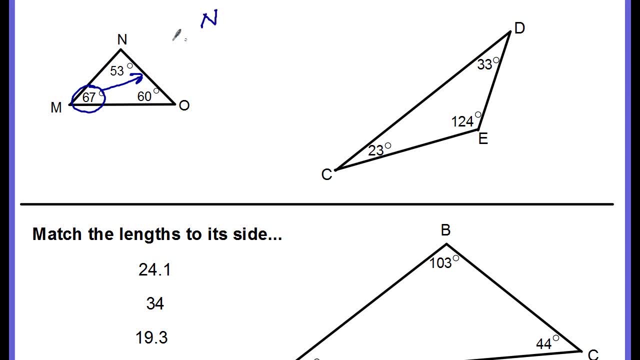 So the way you write the sides is you write it with the letters NO and then you put a line above it. You could also write it as ON. the order doesn't matter for a side, But this is going to be the longest angle. 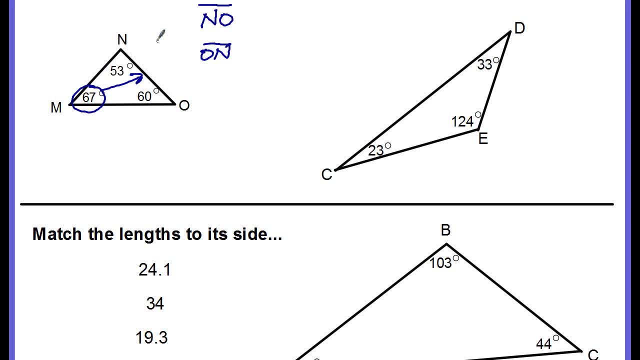 This is going to be the longest or the shortest. I'm sorry, this is going to be the longest. Okay, now let's go with the middle. The middle degree is the 60 degrees, which is angle O And which side does not touch it. 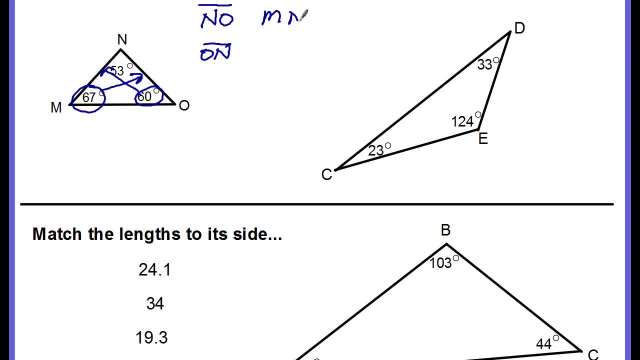 This MN side, So MN, which can also be written as NM. make sure you put the line above. it is going to be the middle And then the smallest angle is 53.. And the side opposite it is the MO, because it doesn't touch it. 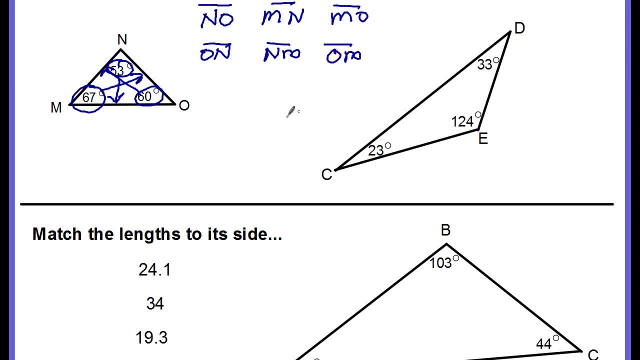 So you could say MO or you could say OM, And this is the largest to smallest order. Again, you can write it either way. Go ahead and try the next one. Put the sides in order from longest to shortest. Once you have your answer, come back and check your work. 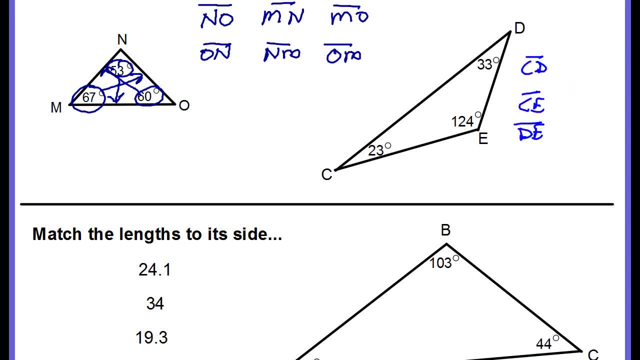 Okay, let's see how you did: Longest to shortest. The longest side is CD. 124 degrees is the largest angle, so the longest side is opposite And that would be side CD, or you could say DC. Okay, next would be CE. 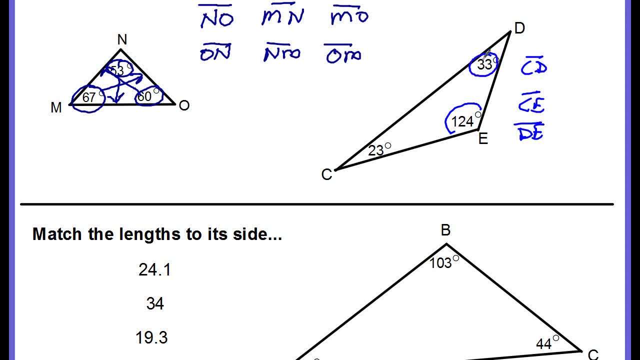 The next largest angle is this: 33 degrees angle D. The side opposite is CE, or you could say EC, Which means the shortest side is opposite the smallest angle, which would be DE or you could say ED. How'd you do? Okay, now we're going to match the lengths to its side. 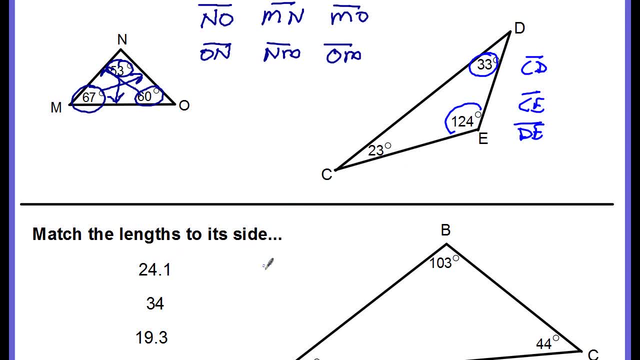 We're basically doing the same thing, except for you're going to write the lengths on the model. Okay, so here we go. Largest. Largest is 103 degrees. That's the largest angle. Which side is opposite the 103 degree or opposite angle B? 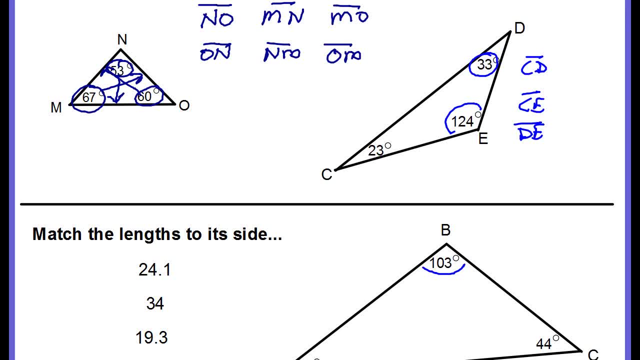 That would be side AC. So when you go to write the length, you write it on the side. Okay, Just like this. A lot of students write it right next to the letters. Nope, We're identifying the side, So it goes on the side. 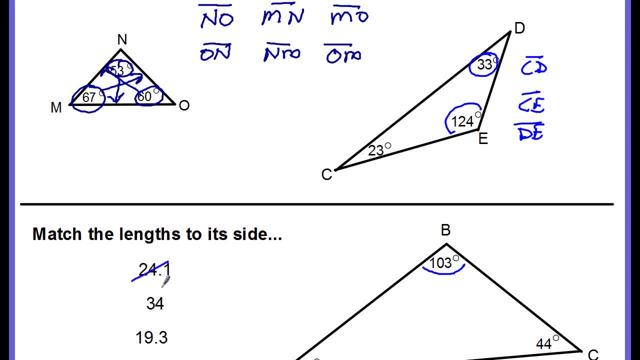 Not in an angle, not by an angle, And that was wrong. Did you guys catch my mistake? Sorry about that. The longest side is not 24.1, it's actually 34. So the 34 goes here, Okay. 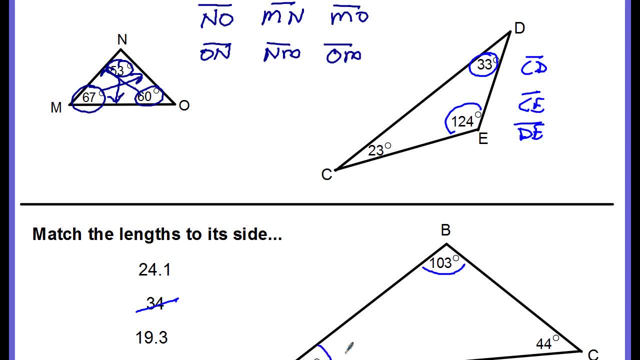 So what is going to go on the side opposite, 34?? Go ahead and write it. Since 34 is the smallest angle, then the smallest side, the 19.3, would go opposite it, Which means that the middle angle 44 degrees the side opposite, that would be the middle. 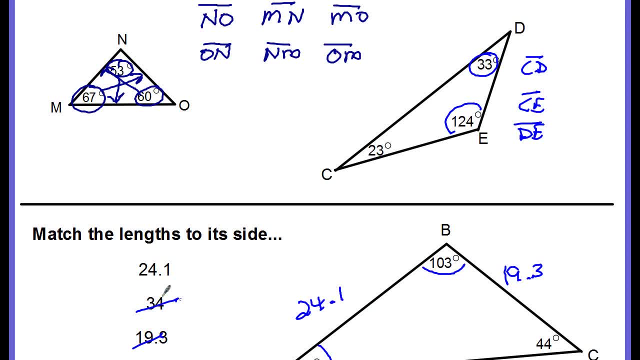 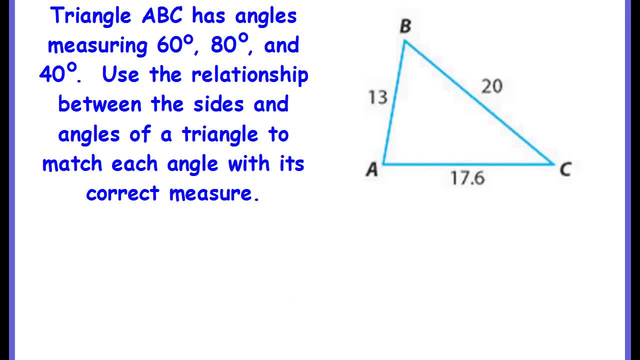 sized side, which is 24.1.. Okay, Now we're going to look at it being given the side lengths and we're going to have to figure out where the angle degrees go. So triangle ABC has angles measuring 60 degrees, 80 degrees and 40. 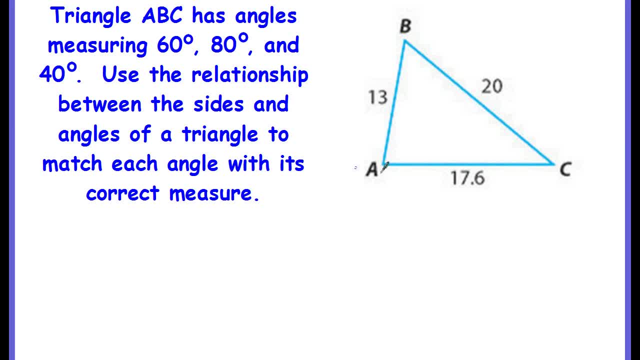 Use the relationship between the sides and angles of a triangle to match each angle with its correct measure. Okay, We're doing the same thing. Large goes. large is opposite large, Medium is opposite medium, Small is opposite the small. So we'll start with the largest side. 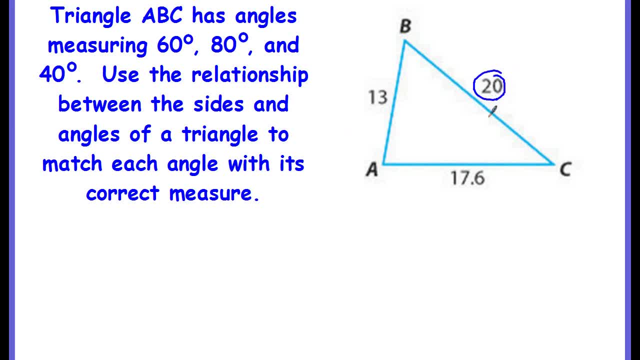 We're going to start with the largest side, Which is 20.. And I need to go to its angle. So which vertex does 20, this side not touch? It touches the B vertex and it touches the C. It does not touch the A, That means the. 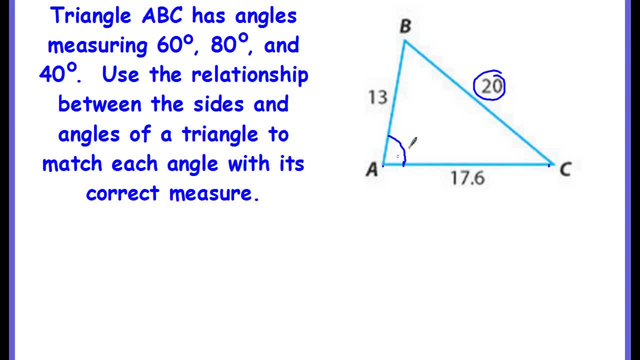 angle A, vertex A is opposite the 20.. Since 20 is the largest, angle A is the largest, which would be 80 degrees. Okay, Let's go with the smallest, The smallest side. The smallest side is side AB. 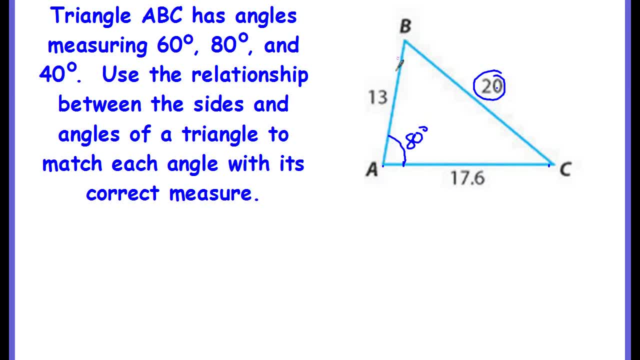 Which side is opposite, or which angle is opposite. Well, it's going to be the vertex that this side does not touch. It does not touch angle C, So angle C is opposite the 13. This is the smallest size, so angle C is the smallest angle, which is 40 degrees. 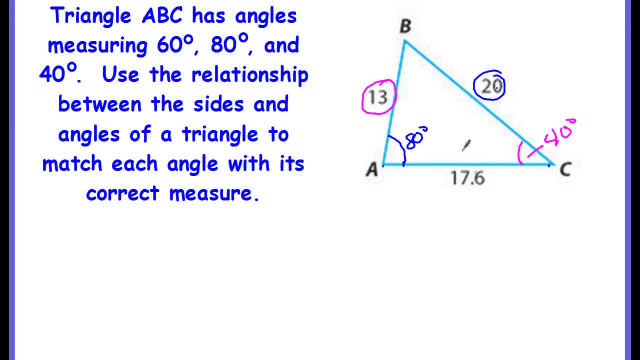 And that means that the middle side, 17 and 6 tenths, is opposite angle B. So angle C- 17 and 6 tenths- is opposite angle B, So angle C is the smallest angle, which is 40 degrees. 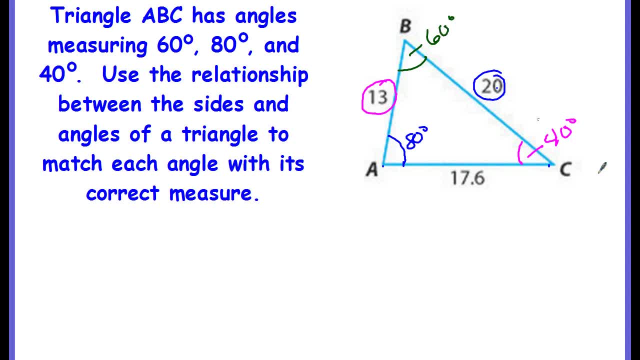 So this would be the middle angle, which is 60 degrees.